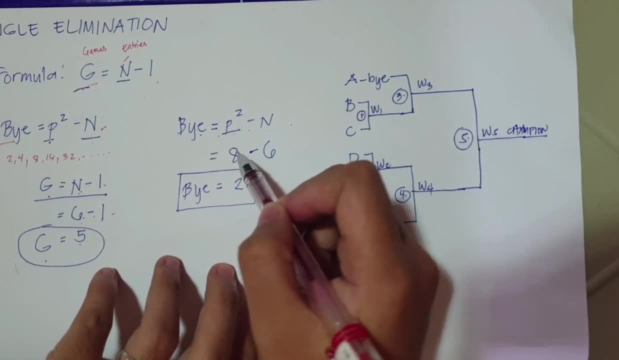 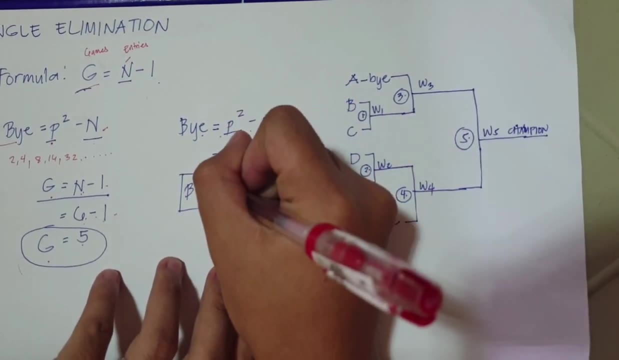 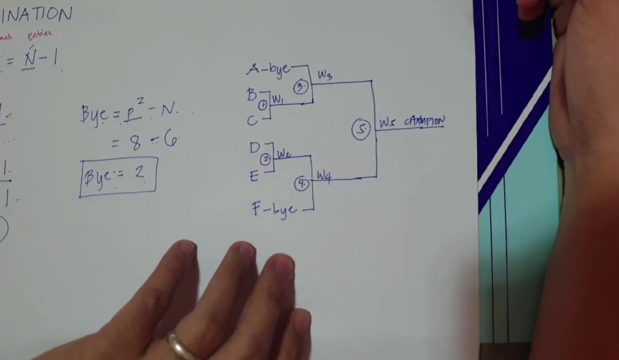 So we are going to replace p squared with 8, then minus 6 number of entries, So there are 2 buys in 6 participating teams Now in making the diagram. so first step is we are going to assign letters to the teams. 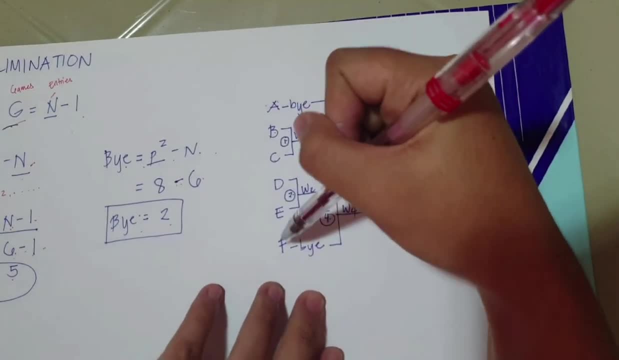 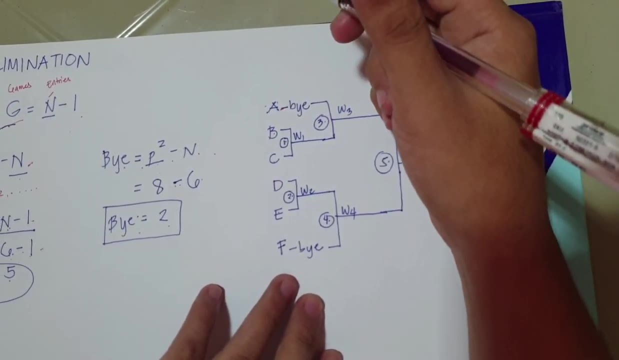 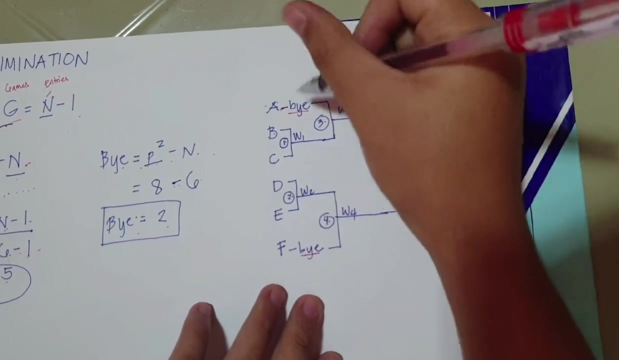 So let's say, for example, team A, B, C, D, E, F. Next step is we are going to assign what particular team ang atuang himoong buy. So let's say, for example, A and F, so sila ang buy. 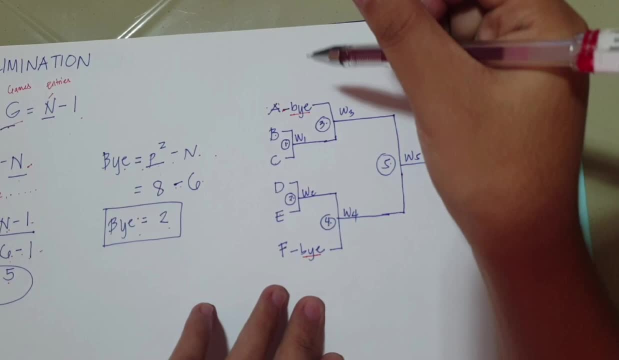 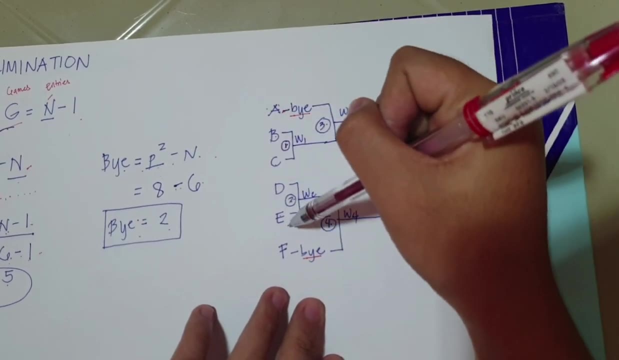 Okay, Next step we are going to choose kinsaang magdula for the first game and second game for the first round. So this part here is the first round. Next here is the second round and then the final round. Okay, 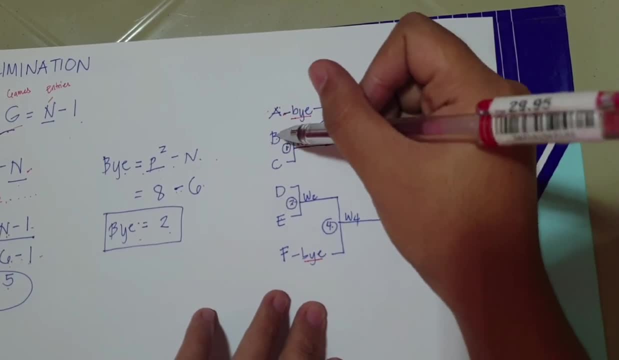 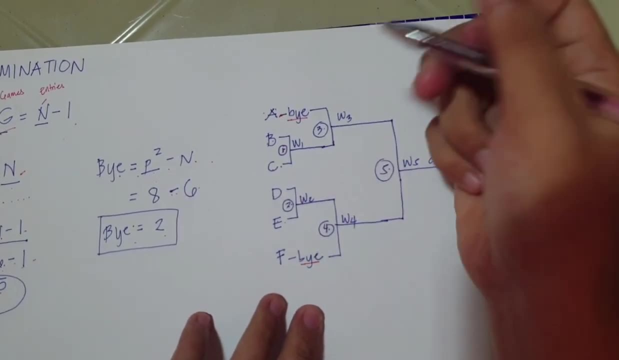 So for the first round, I'm going to choose, for the first game, team B versus C and then for the second game, team D and E. Okay, So after the game, we are going to declare who will buy, Who will be the winner for the game 1 and 2.. 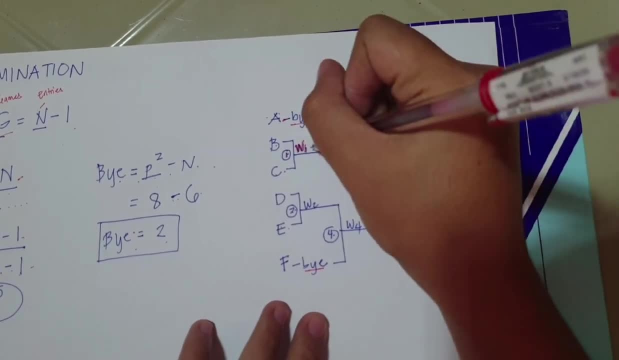 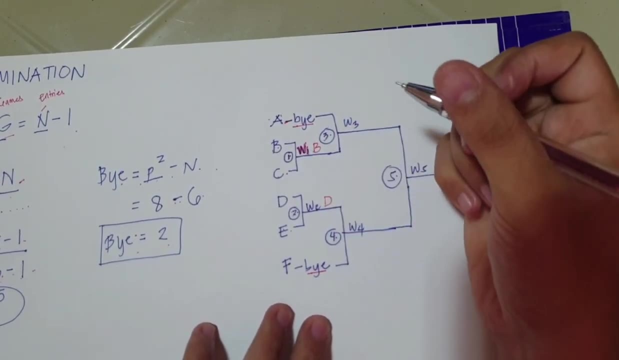 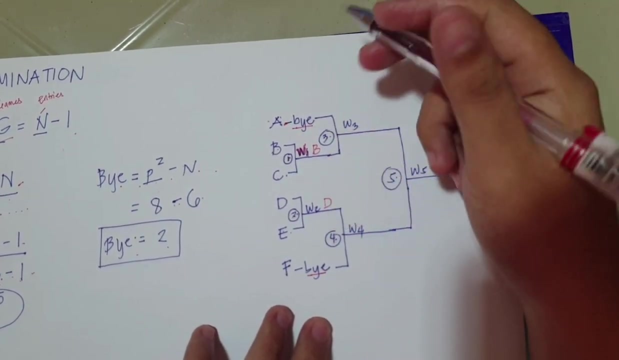 So let's say, for example, for the winner: 1 okay, letter B, ang winner. and then for the game: 2 si letter D: Okay, Now for the second round. so since team A and F ang nadeclare nga buy, so we are going to. 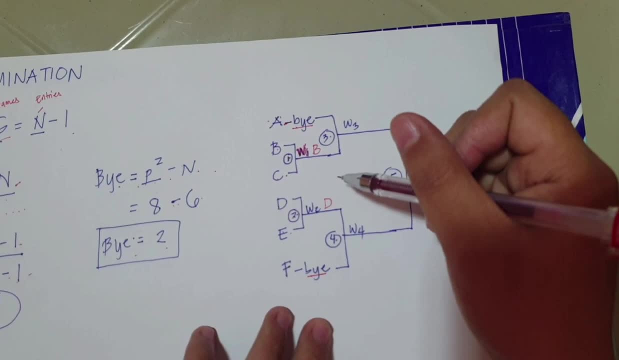 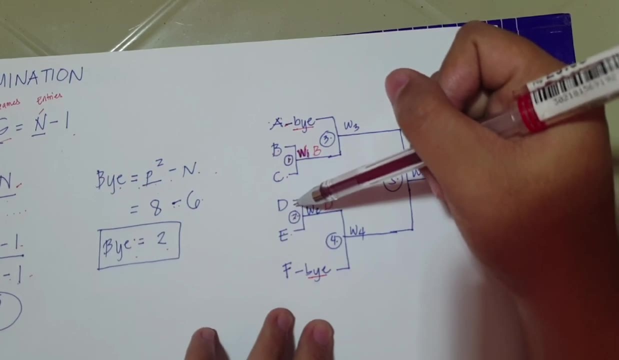 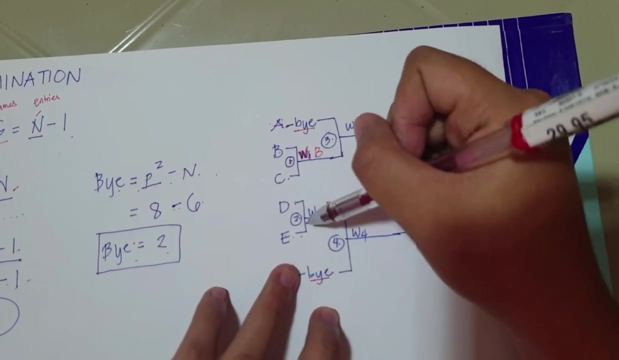 assign na naman who will be the team nga magplay for the third game and fourth game. So for the first round. so ang last nga nagdula is si team D and A. no, So next is: so since si D and E ang last nga nagdula, make sure nga ang sa next round nga. 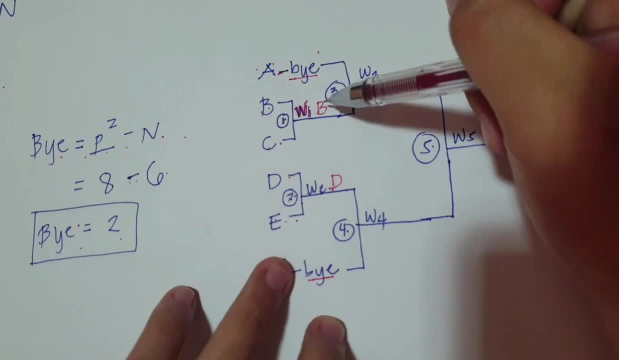 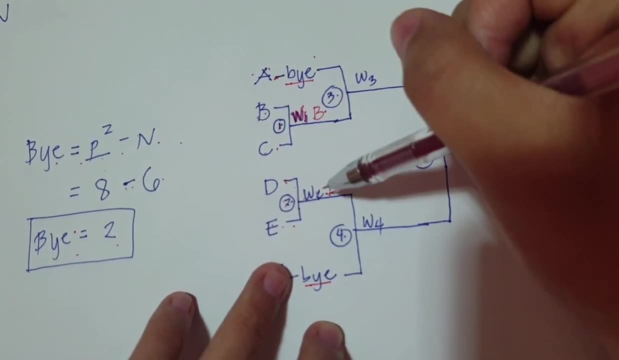 magdula is si letter A and B, since katatapos lang man ni D and E nga magdula, so na pa siya time nga mag rest, So ato ang i-assign nga for the third game is si letter A, Okay.